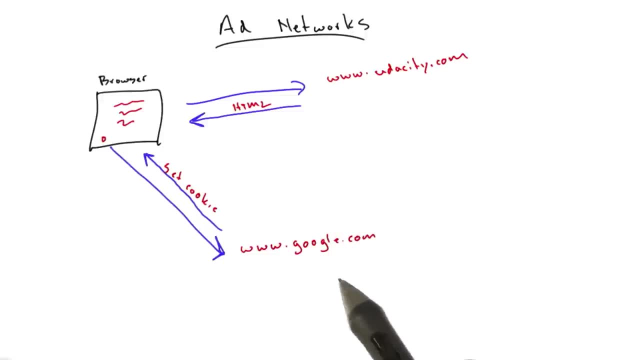 And you know that. you know that's how they know whether you're a new user or a returning user, And and so this is. you know this is an example of of a third party cookie. You know we went to udacitycom in our browser. 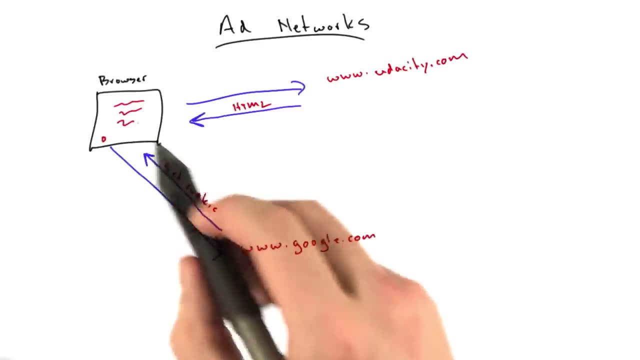 But we received a cookie for googlecom. You know, Udacity doesn't receive those cookies, but Google will, And and that's how they run their analytics, And and there are legitimate uses for this. You know, analytics is a really good example. 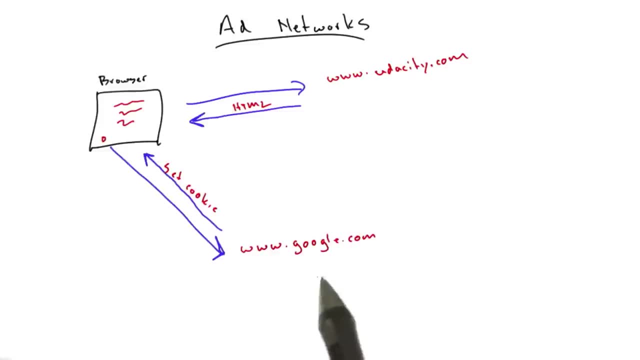 We, you know we use Google Analytics on. you know we used it on Reddit and we use it currently on Hipmunk, and Udacity uses Google Analytics as well. So we can see, you know what our traffic is, what people are clicking on. 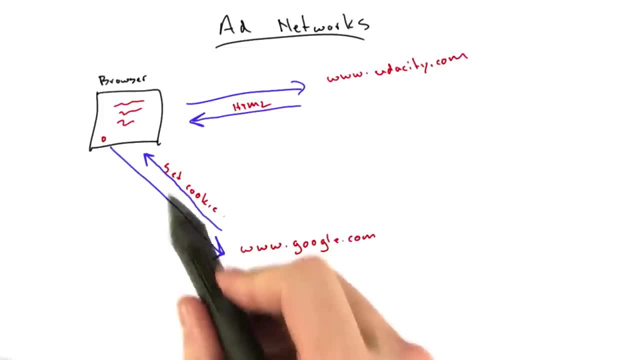 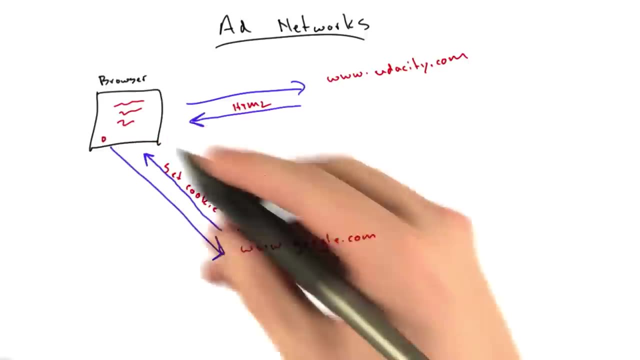 that sort of thing. There's also more sinister uses, which is actually. Google is a big user of this. Now, Google knows something about you. You know. they know that you've been to this website And you may go to another website. 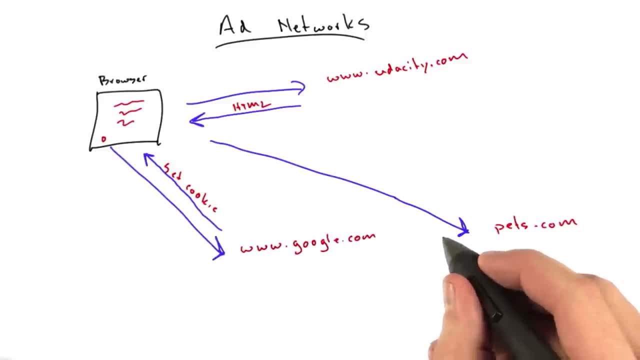 You know, let's say it's, it's petscom, And petscom, you know, returns HTML, you know, as usual, And it has the same pixel which goes to googlecom. All of a sudden, Google knows. hey, you've been. 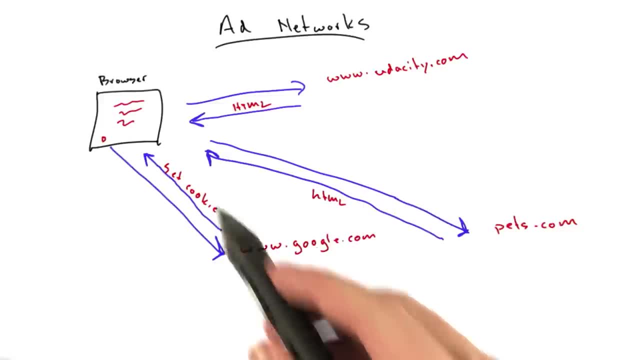 to udacitycom and petscom because they're like a common third party here And Google actually has, you know, between Google Analytics and and AdSense and that sort of thing. they actually have pixels and and a presence on a huge percentage of web pages. 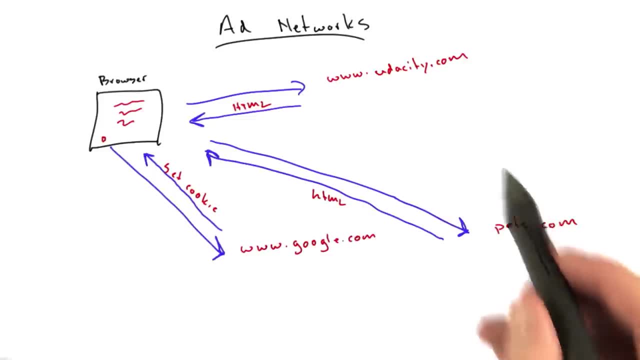 You know they have this one of the largest ad networks, And so now they know this information and they can. they can give you ads that are more relevant to you, Which is sometimes you know you. you can argue that both ways. 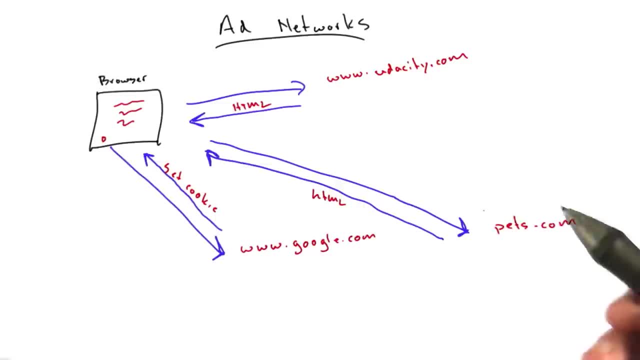 You can say, oh, that ad's more relevant to me, You know, so I'm more likely to click on it. Maybe that's a good thing, Or it's creepy that this company knows all these different websites I've been to. 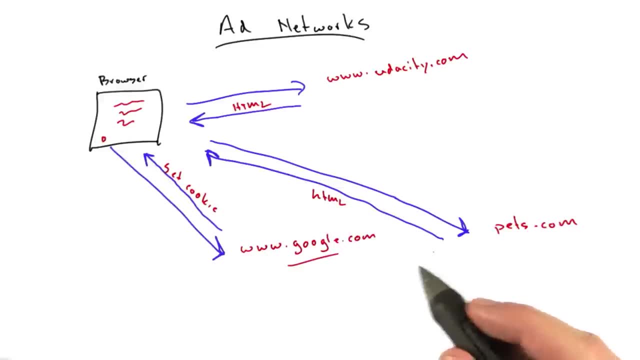 Now, generally we can trust Google, but you can't say the same for all all ad networks. So anyway, that's kind of how they work. They've got these little tracking pixels And when you disable third party cookies in your browser, 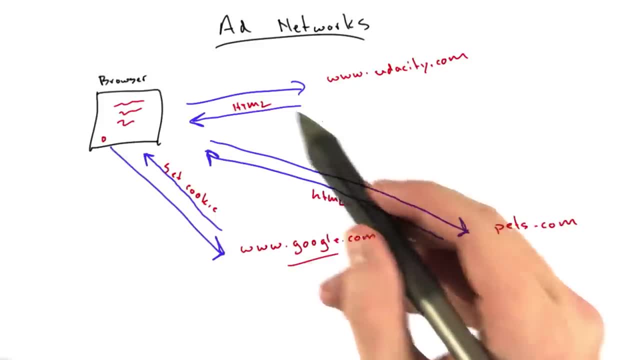 you help disconnect yourself a little bit from from that sort of tracking. And you know I don't mean to pick on Google specifically, because you know they're actually, you know, not too shady, But there are a lot of shady variations of this out there. So that's how it works.